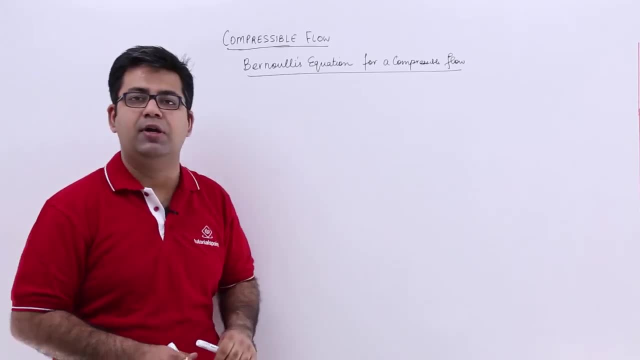 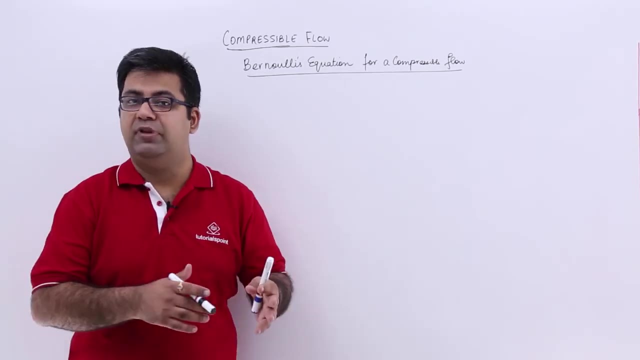 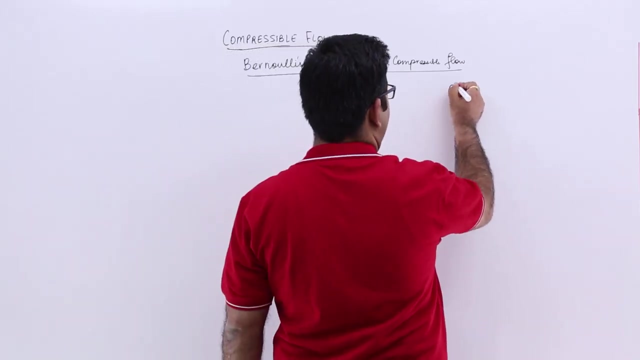 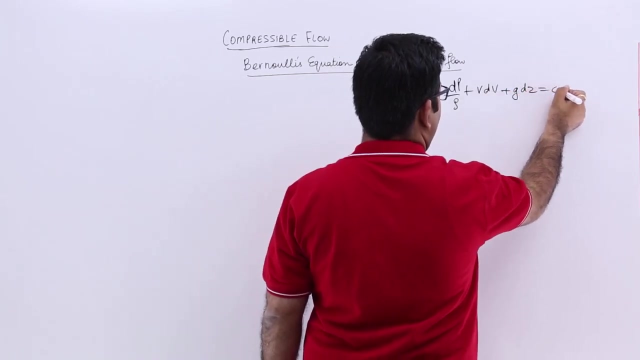 Now let's talk about the Bernoulli's equation for a compressible flow. Now, Bernoulli's equation is an equation which is a result of the integration of the Euler's equation. So Euler's equation for an incompressible flow was this: dp upon rho plus v into dv, plus g into dz is equal. 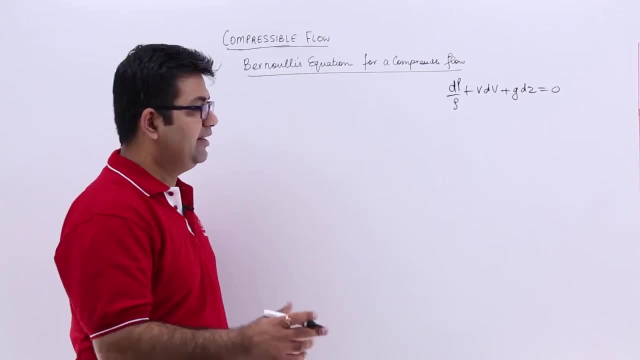 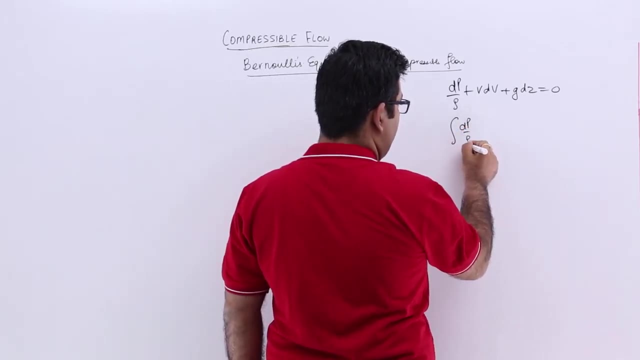 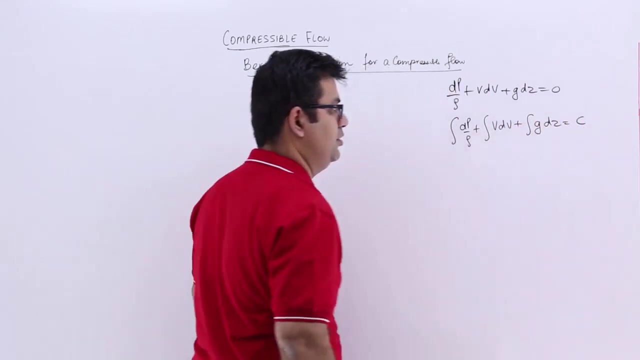 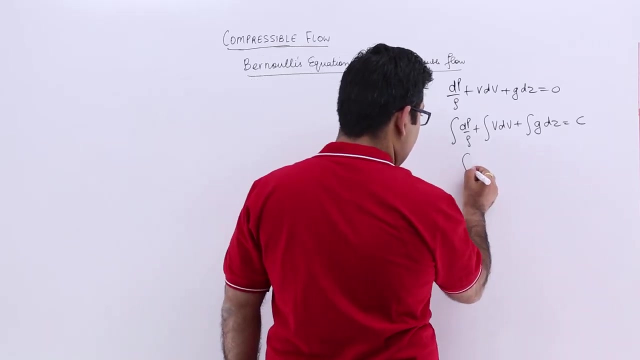 to 0.. So this is the Euler's equation. If I integrate this, I get Bernoulli's equation, So you will get integral dp upon rho plus integral v. dv plus integral g into dz is equal to constant. This will give you the Bernoulli's equation, So you will have integral dp upon. 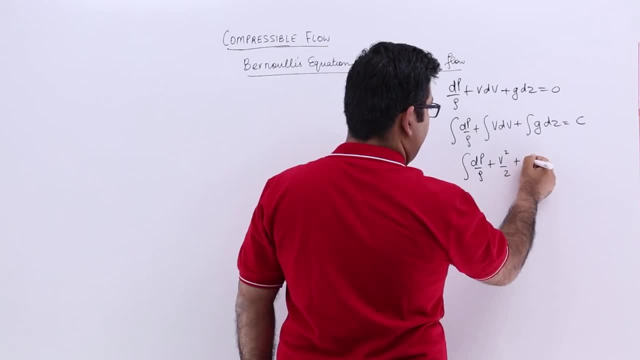 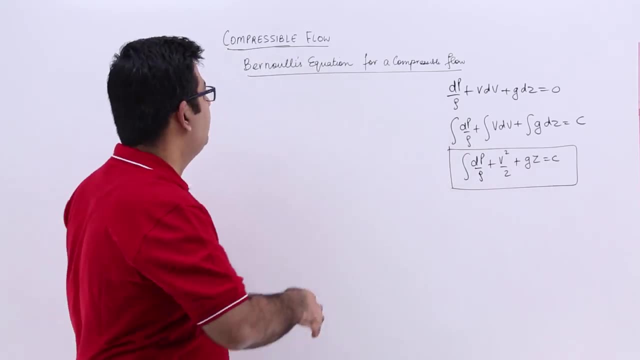 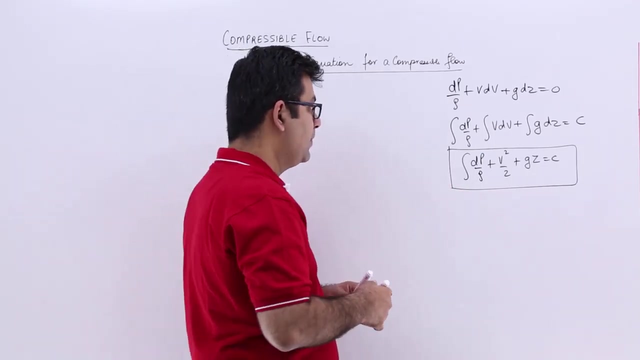 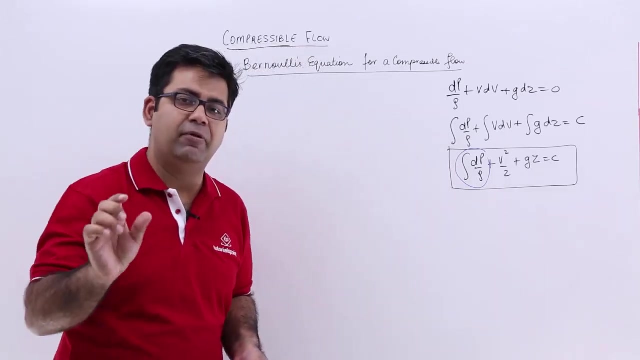 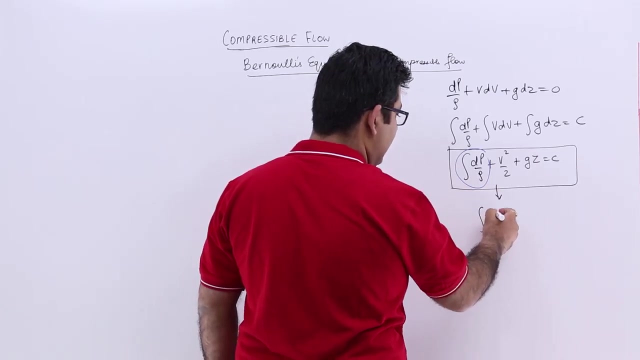 rho plus v square upon 2.. Okay, So the entire difference between the Bernoulli's equation for a compressible flow and for an incompressible flow falls upon this term, That is, integral dp upon rho. Okay, For an incompressible flow when rho is a constant value, then we can say that integral dp upon 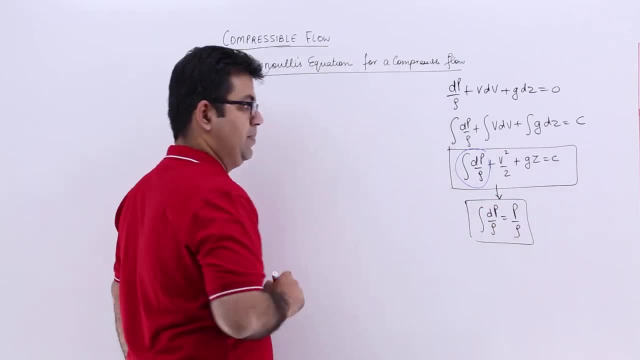 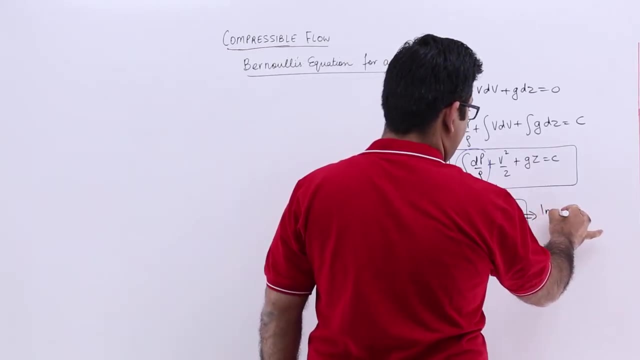 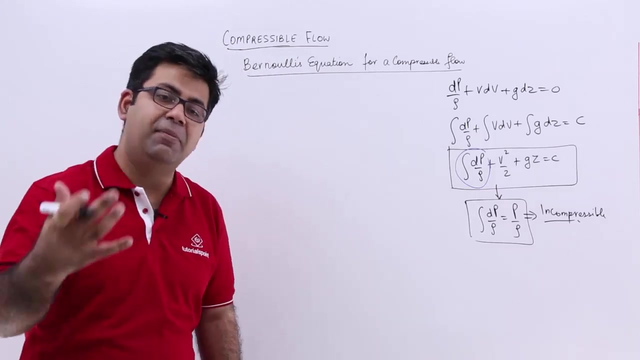 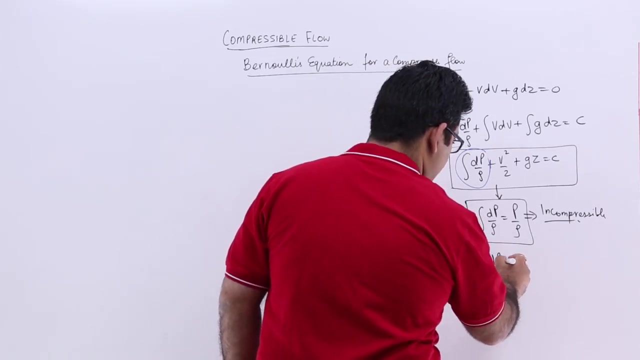 rho is equivalent to p upon rho because the value of rho is constant. So this is for an incompressible flow. Okay, But for a compressible flow this equality is not valid. means that integral dp upon rho is not equal to p upon rho. Okay, 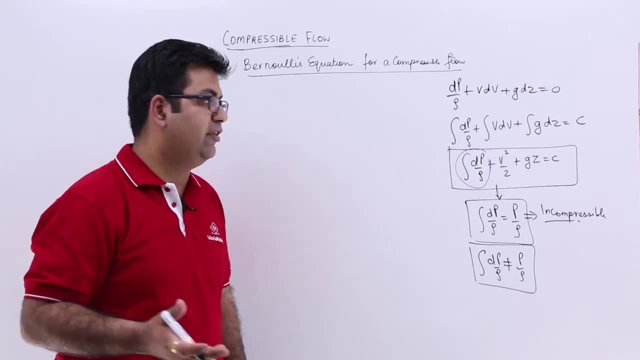 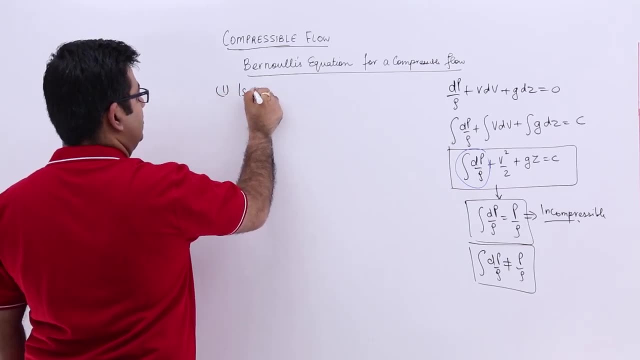 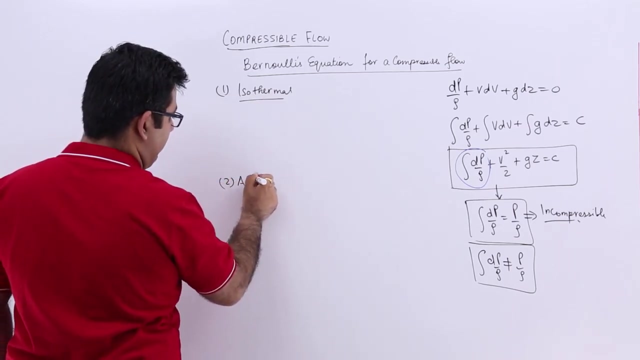 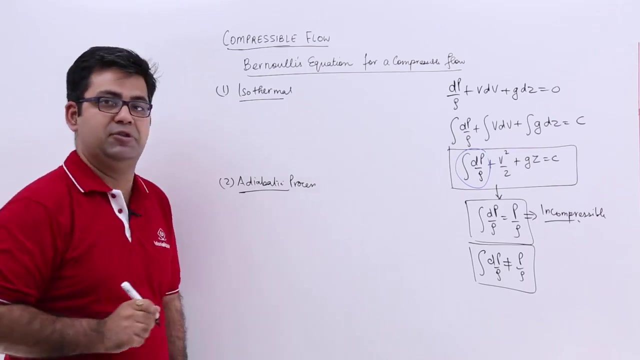 So again, there are two processes for which we define the Bernoulli equation for a compressible flow. The first one is an isothermal process and the second one is an adiabatic process. Okay, so let's look at the very first one, that is, the isothermal process. 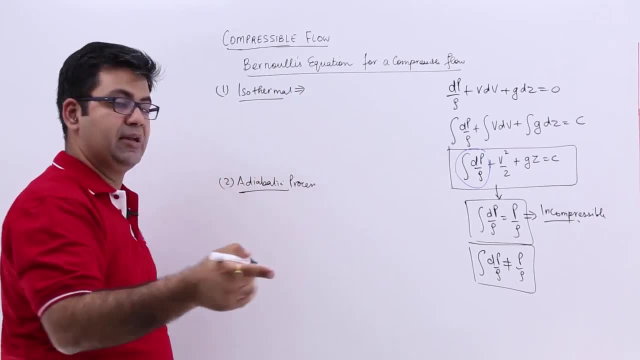 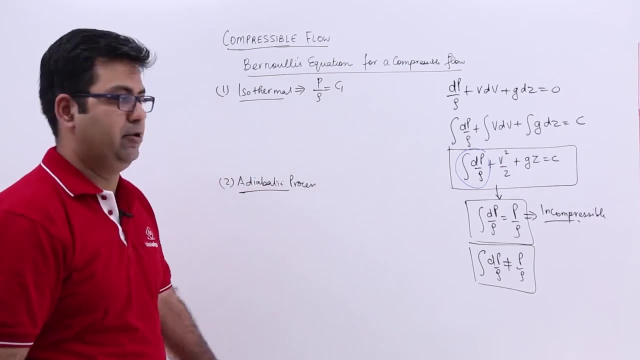 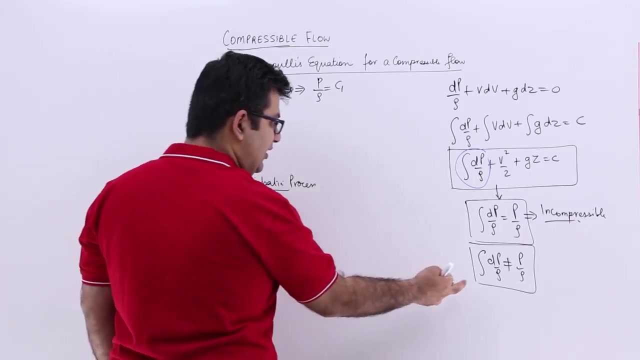 The relationship between the pressure and the density for an isothermal process is this: that p upon rho is equal to a constant, that is a C1, because we have already used C. Okay, so this is the isothermal process. So to evaluate this integral- because rest, everything is resolved- I need to get a value. 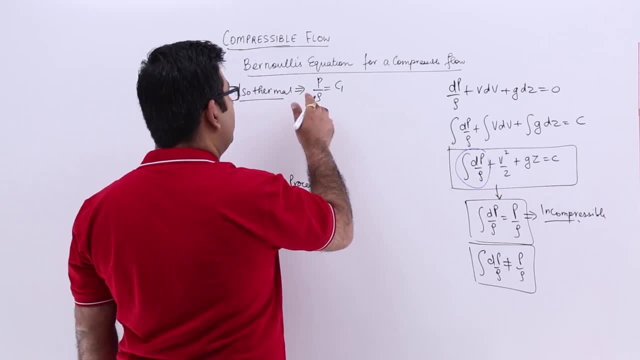 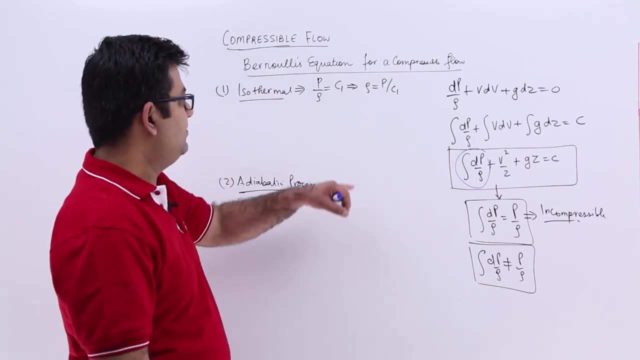 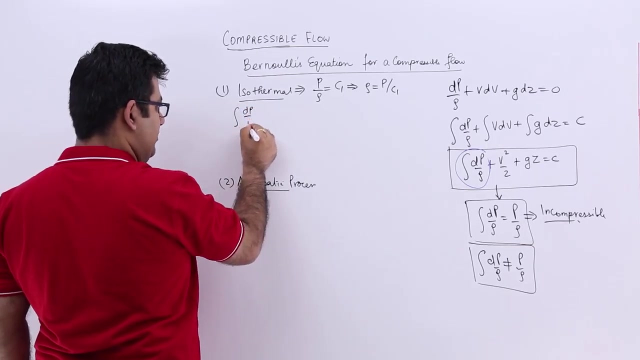 for dp by rho integral. I need to get a value of rho from here, So the value of rho will be equal to p upon dp by rho. Let us substitute this rho into this equation or that integral, so you will get dp upon p into C1. 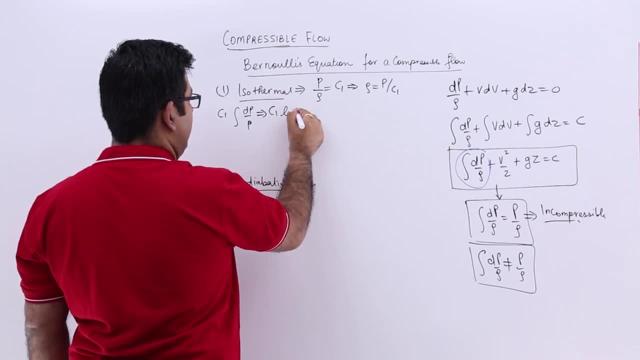 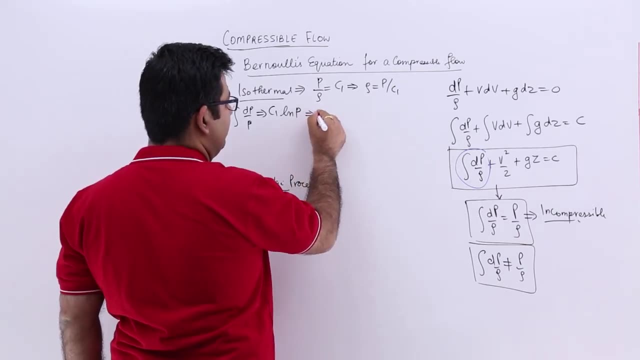 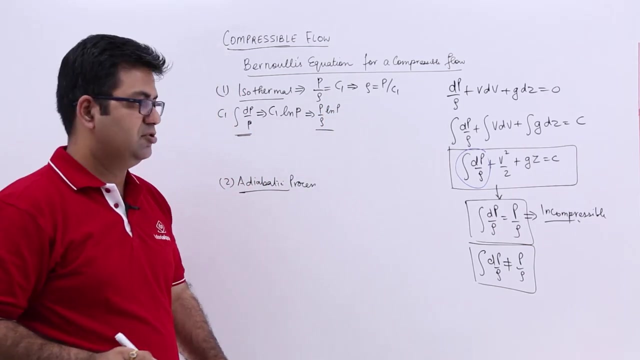 So this would be C1 into natural log p. What is C1?? C1 is p upon rho. So finally, I will get a value which is p upon rho into natural log p. So this integral is dp by rho. Okay, So this integral is this: 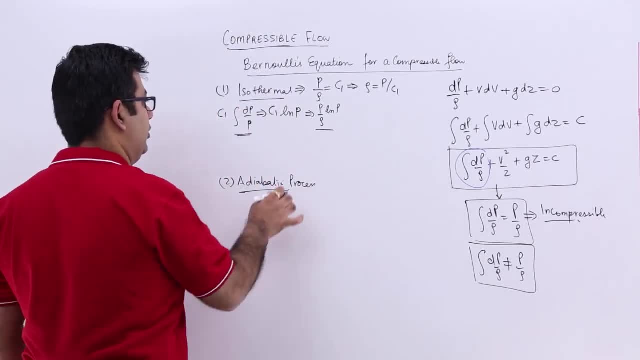 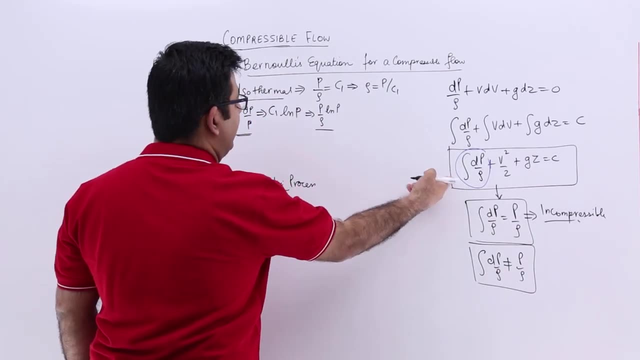 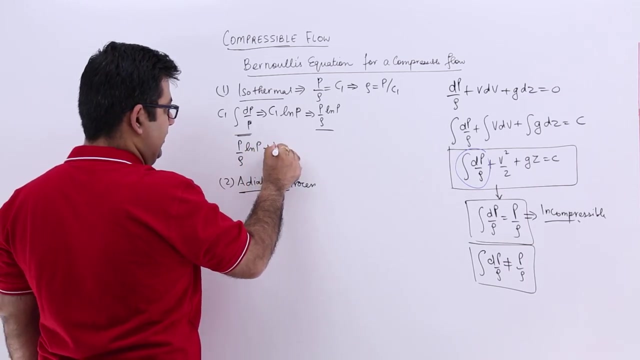 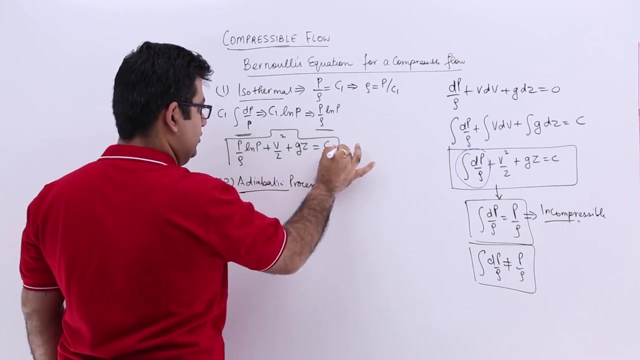 So the Bernoulli's equation for the isothermal process, which is for an incompressible flow, will become so. in this place I will write: p by rho log p, p by rho natural log p plus v. square by 2 plus g into z is equal to constant. 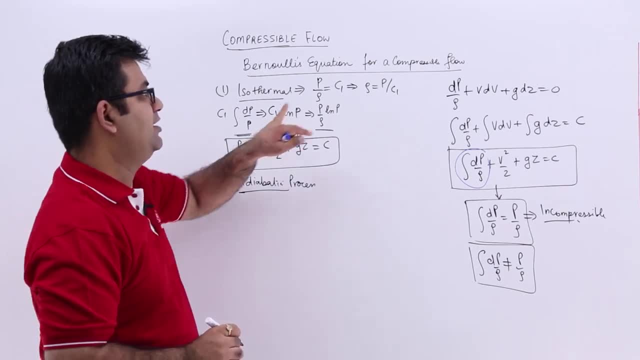 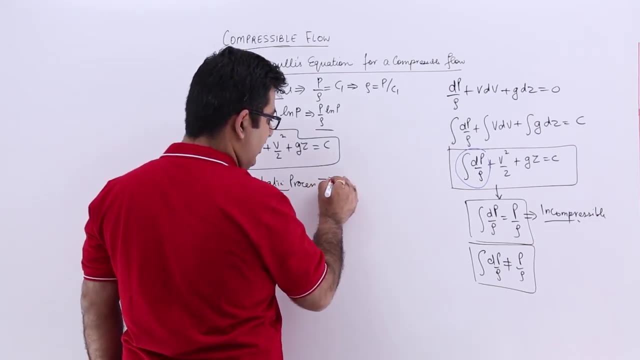 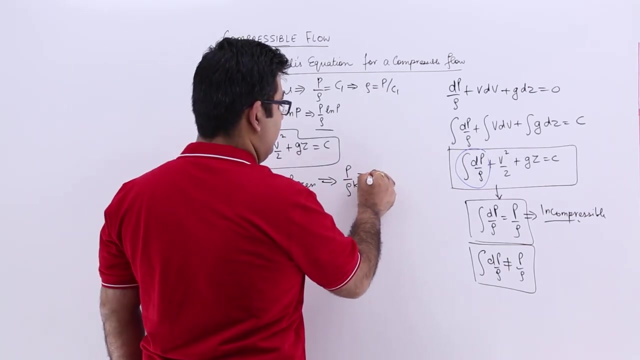 So this is the Bernoulli's equation. Okay, For a compressible isothermal flow. Now let us look at the adiabatic process. The governing law for the adiabatic process is this: P by rho to the power, k is equal to a constant. let us say C2.. 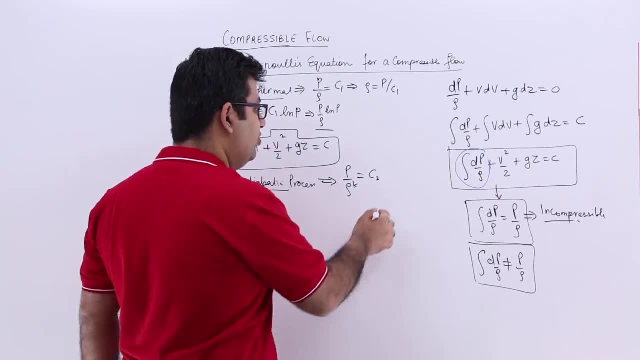 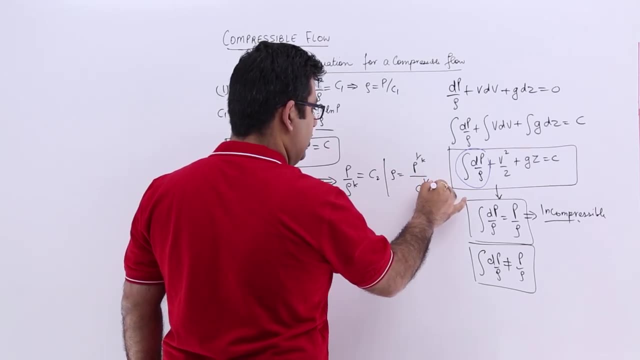 So again, I need to get a value of rho from here. So the value of rho will come out to be p to the power 1 by k upon C2 to the power 1 by k. Okay, Let us put this into that integral. 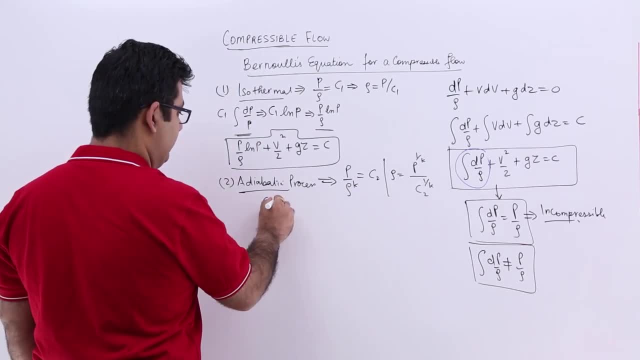 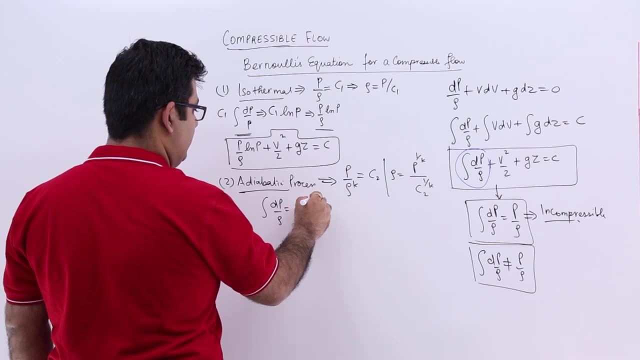 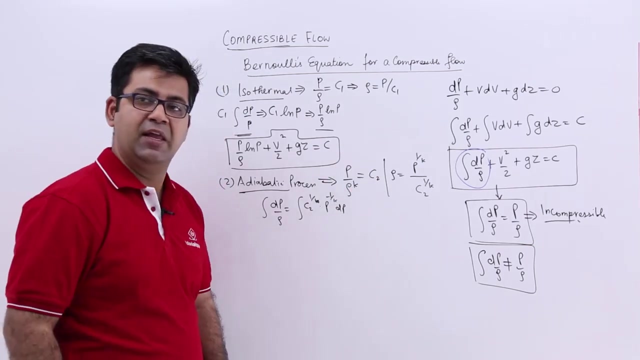 So you will have integral dp upon rho is equal to integral C2, to the power 1 by k into p, to the power minus 1 by k. dp- This is the constant value- can come out of the integral sign and you will have C2.. 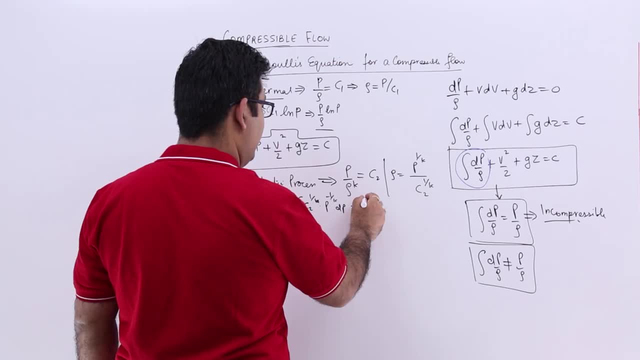 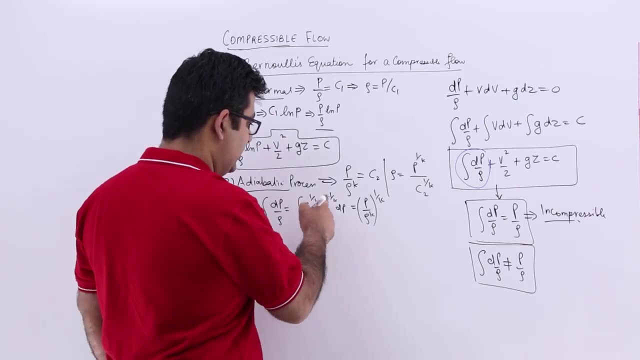 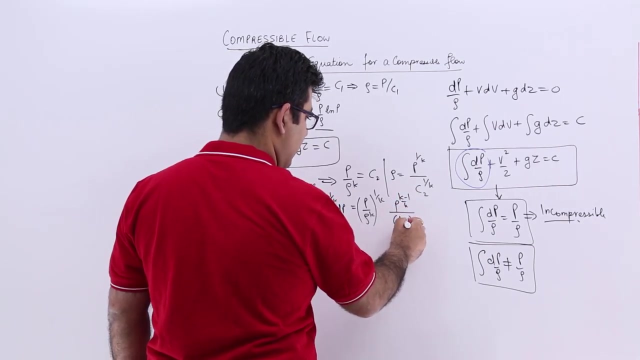 How much is C2? p by rho k? You will have p upon rho, Okay. So rho to the power k whole to the power 1 by k, Okay, And this integral would be p to the power k minus 1 by k upon k minus 1 by k.